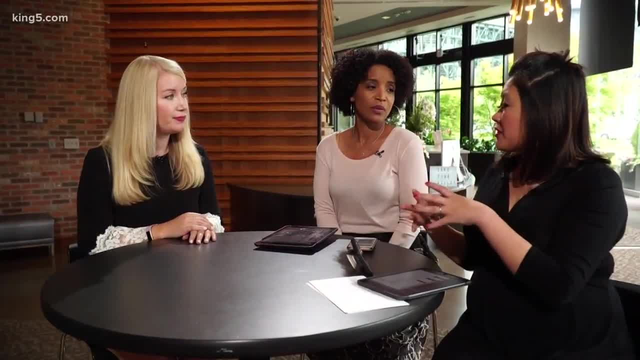 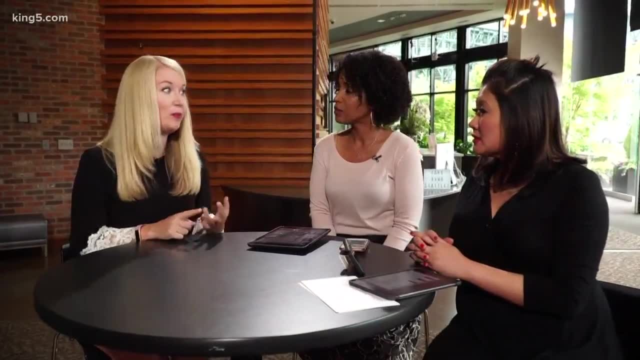 Well, and that begs the question, because I know people with who are vulnerable, Right? So you're talking about babies, maybe seniors or the elderly, Babies, pregnant women, people with immune problems, immunocompromised- they're all at risk, if they get measles, of getting very, very sick or even dying. And you can't get a shot, right Like you can't get the vaccine when you're like a brand new baby. You have to wait a while, Yeah, So typically it's at 12 to 15 months, and then the second dose is four to six years. There are certain circumstances: if someone's traveling to a country with really high rates, we may do it a little bit sooner in infants, but very young infants aren't able to get the vaccine. 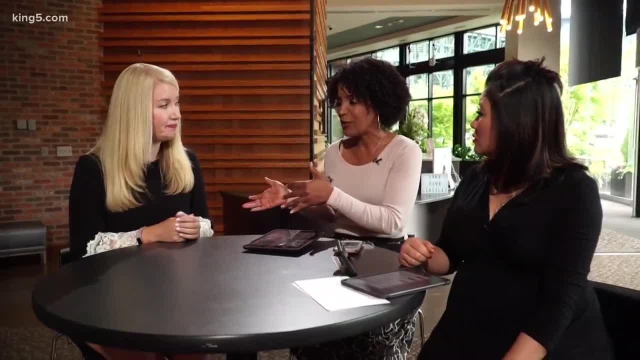 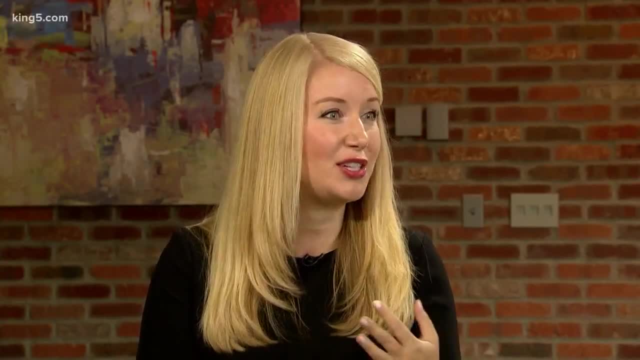 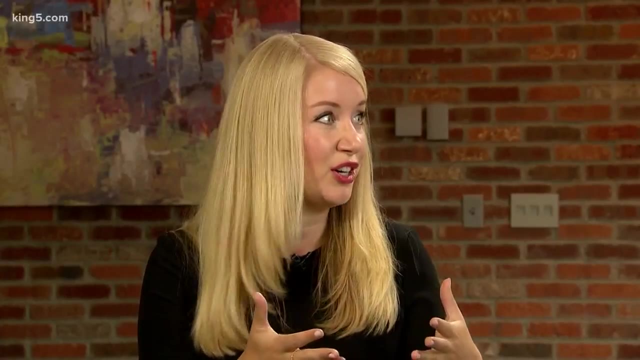 So if someone doesn't get it, or parents don't have their children get it, they could be putting at risk infants who are not- Oh, so they're old enough to get that vaccination- Absolutely Infants, or people who can't get it. So some people who have cancer or immune problems aren't able to get vaccinated. There may be people- there's a very, very small subset of people- who just aren't responders so they don't get the immune, you know, the antibodies, even if they've been vaccinated. 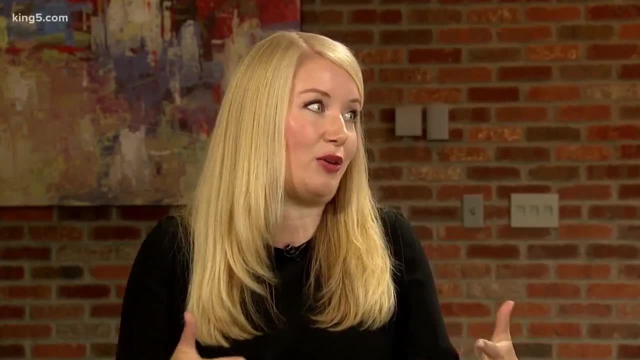 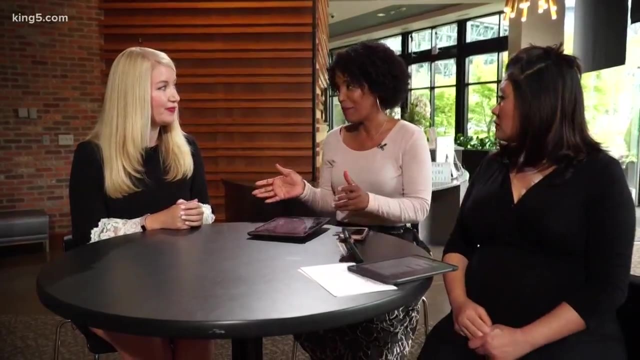 So people who are not vaccinated are absolutely putting those other people at risk who can't get the vaccine, And that's really the concern I see. Yeah, So, wow. So let's talk about this other topic. Sure, You may have been listening. We've been talking about this article that says children should be 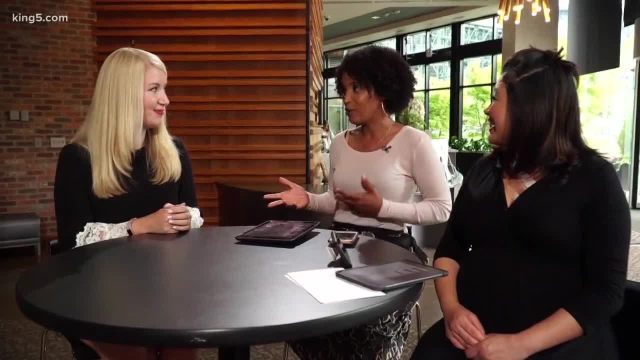 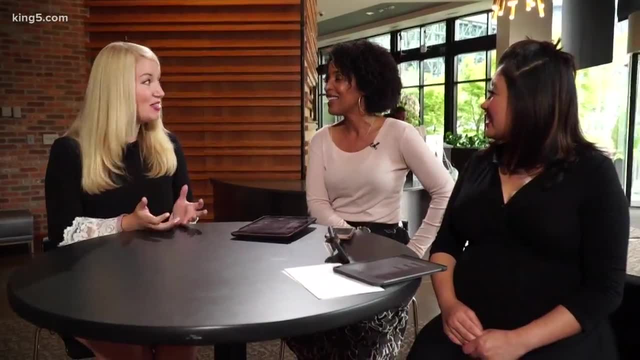 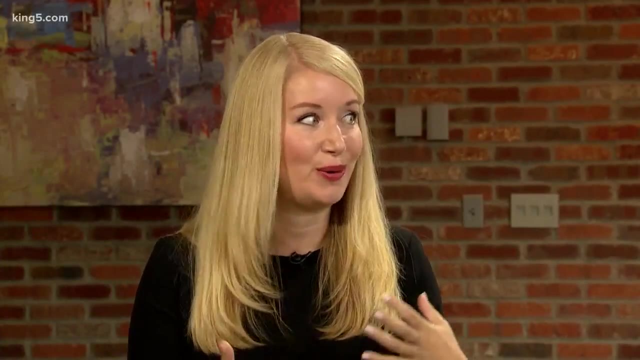 They should be allowed to be bored. And you know you're the head of pediatrics, so, assuming you've spent a lot of time in med school and studying this kind of stuff, what say you on this topic? You know, I do think some boredom is good for kids. I think that kids really need time for creative, imaginative play. They need to use their imagination. They need to come up with their own games. 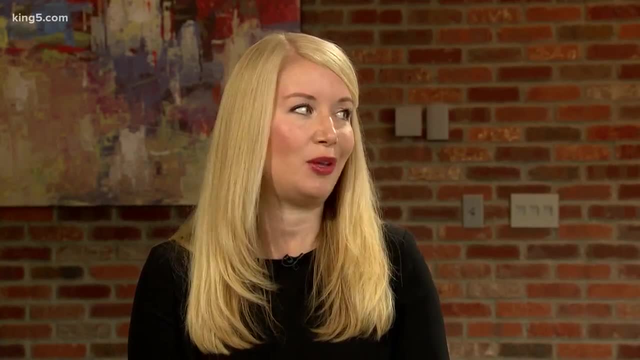 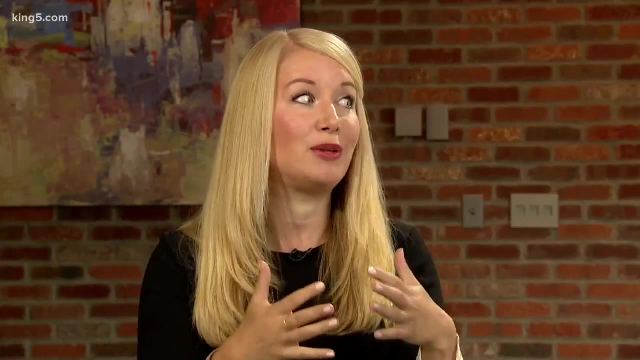 And that's that boredom can kind of spark that in kids, So especially in the summertime. you know we don't want kids sitting around doing nothing all day, every day. But I think some boredom forces kids to not be stimulated by something else all the time and to really have to come up with something. 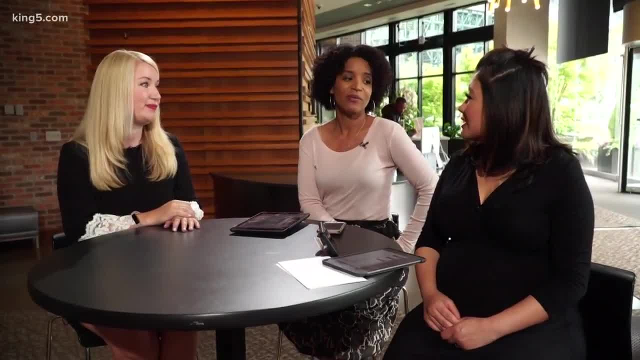 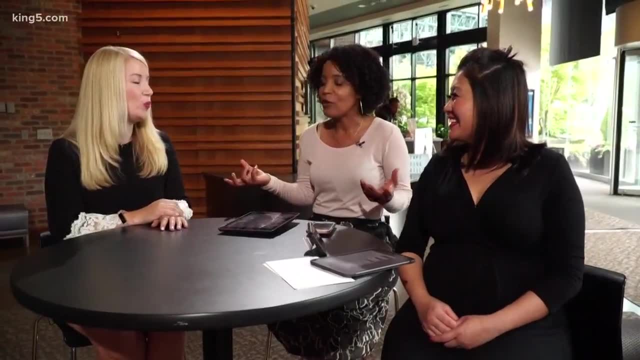 And I think that's a good answer. Not the devil's, The devil's workshop. The idol mind is the devil's workshop. I think there's a balance. right, There's a balance. There's a balance with it. So I don't know, Has anyone ever studied how much boredom is good? Is it like? 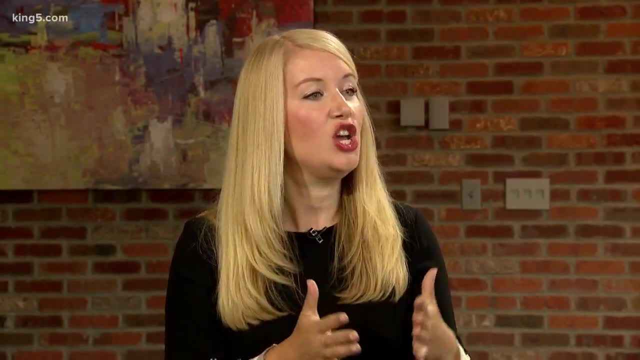 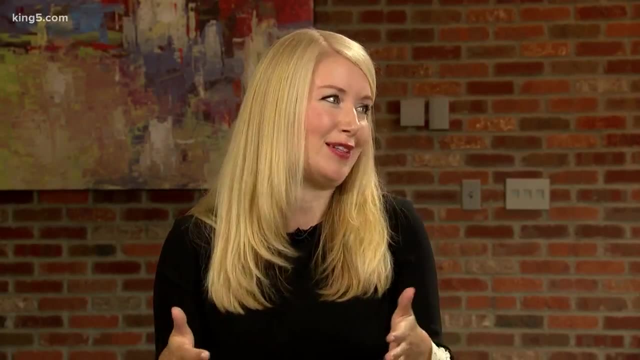 I don't think there's a hard target, unfortunately, that we can go for. But I think you know, if you're noticing that your kids are bored and acting out, behaving inappropriately, talking back, doing things you don't want them to do, then it's probably like okay, that's a little bit too much. 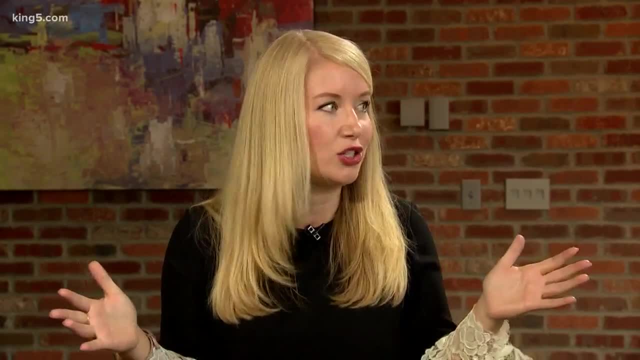 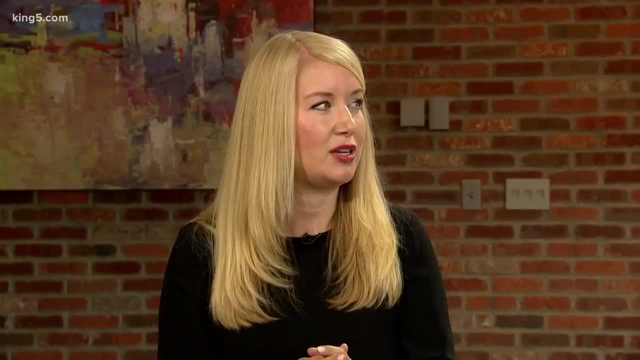 But really the kids need time every day to just have a little unstructured play time Where they're not doing an activity and be able to come up with their own games or read or do whatever they want. So I do think a little bit of it is good to make kids think about what they want to do.